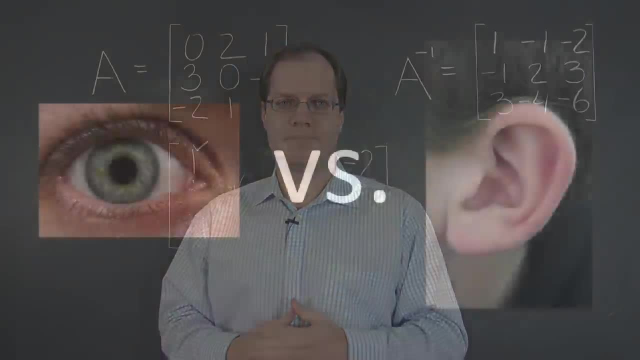 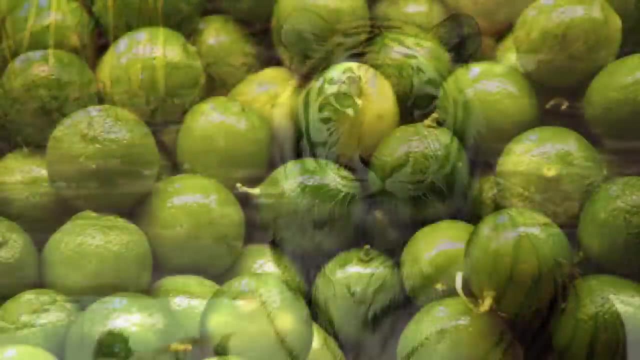 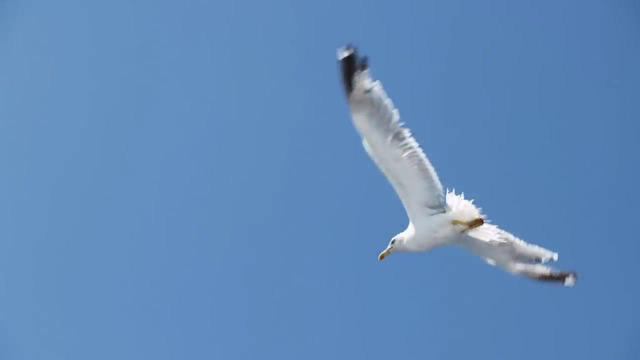 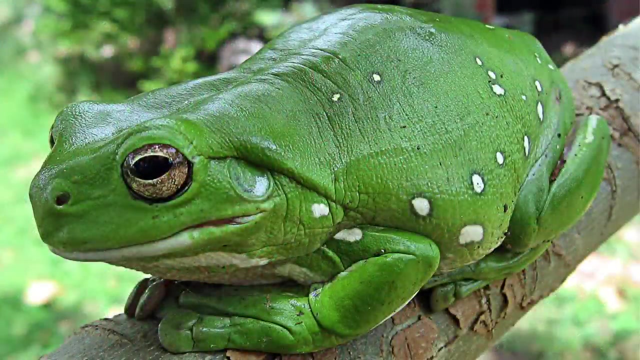 and how our ears perceive sound. You will agree with me that every moment of the day, we have a chance to see something breathtaking. Just look at some of these images. This is possible thanks to one extraordinary organ that we have, and that, of course, is the eye. 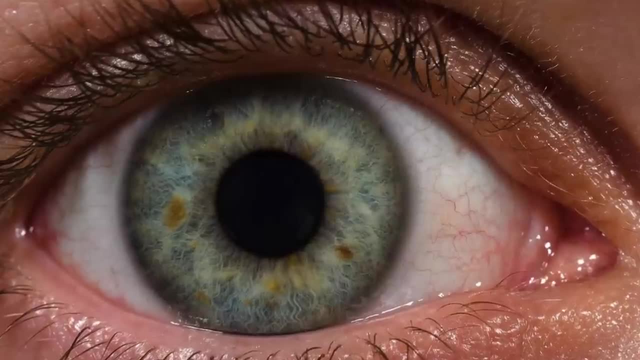 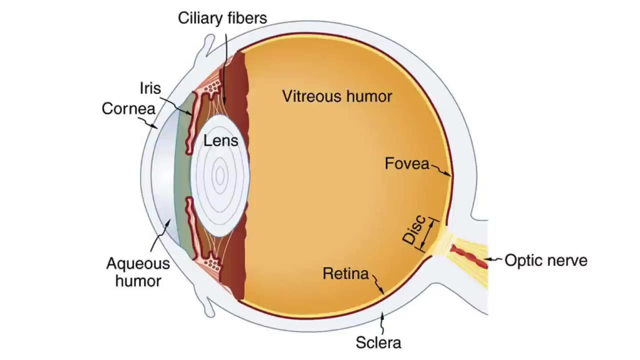 The eye is very complex, to say the least, so we will focus on one particular aspect of one particular part of the eye: the retina, seen in this image as a red line around the perimeter on the inside of the eye. The retina is home to the light sensors. 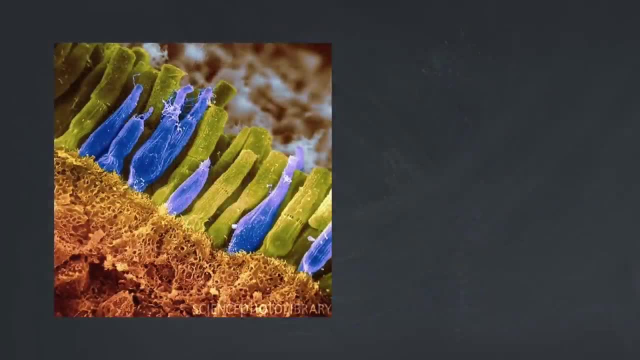 called rods and cones, and it's thanks to their great numbers that we're able to see such striking images. In total, there are around 100 million of them. You can think of this number as the resolution of the eye By comparison, the most advanced monitor today. 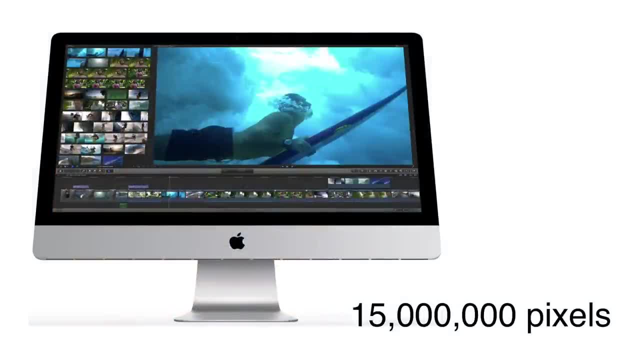 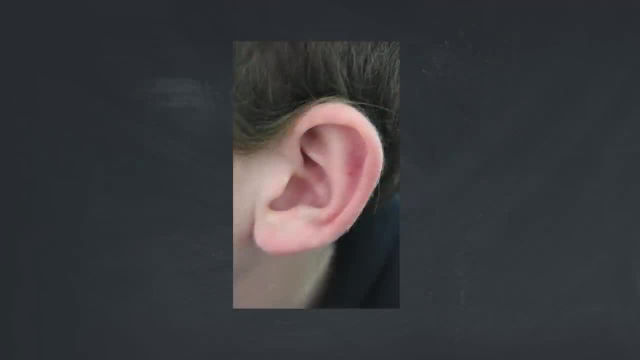 has 15 million pixels, or less than 1 sixth the resolution of the eye. But what about the ear? How many sensors does the ear have that allows it to perceive such beautiful music? Or do you consider the average of theuser as the more complex, the more complex, the more complex? 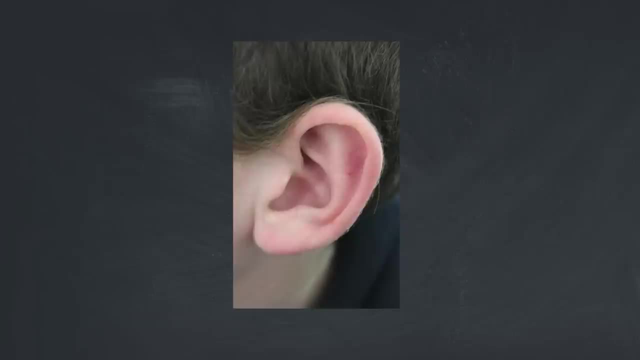 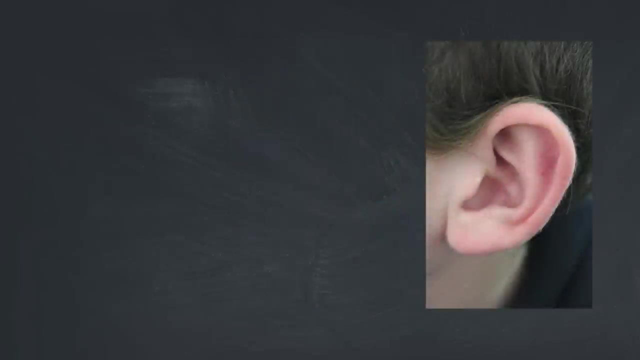 What's the first step to seeing in full detail the most impressive of these images of the eye? Well, this is a very special project because the can be seen as one simple particle that is exactly the same as the eye. Hey, this is an eye, the eye, the eye, the eye. 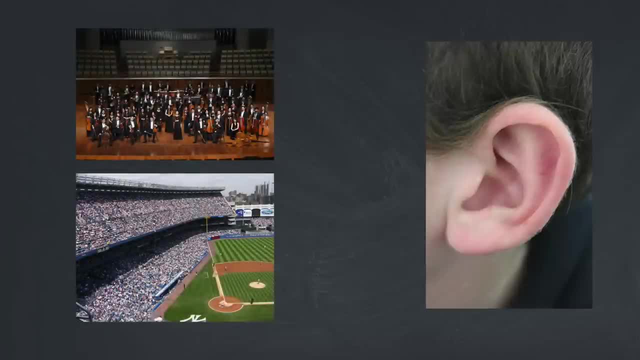 This is a physical, physical body of the eye. The eye is the key to your image, in that it is how we perceive it. Our eyes are like the eye of the human. We believe there are two eyes. Can we see how far the eye is? Can we see how far the eye is? 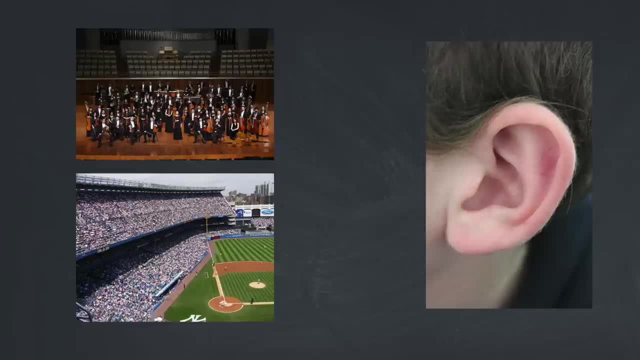 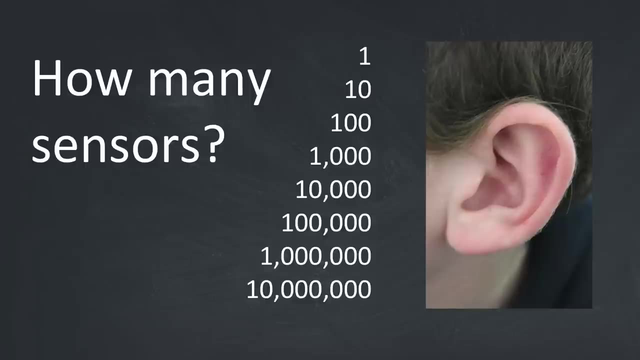 How many sensors does the ear need to take in such complexity? Here, pick the number from the list that you think is about right. The answer might surprise you, because it's one. There is a single signal that enters your ear and it therefore takes a single sensor. 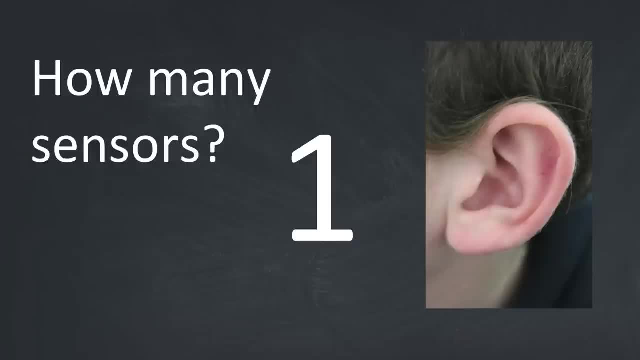 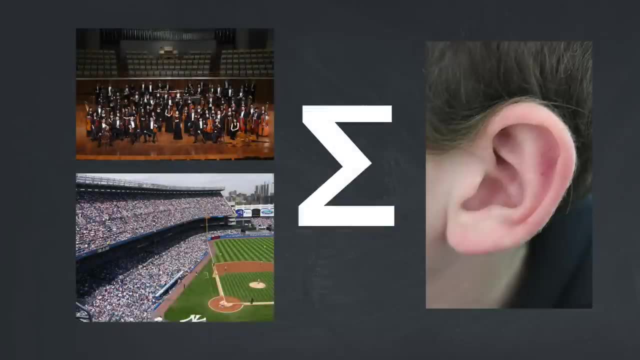 to receive it. Here is what happens: All the sounds simply get added together and it's their sum that enters your ear. But how is that possible? How can one signal contain such richness, And how is your ear able to hear the multiple instruments and voices individually from? 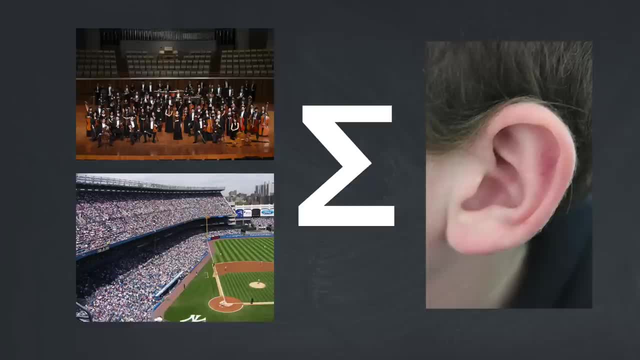 just one signal? Well, this is the mystery that linear algebra will eventually help us solve. Meanwhile, I will show you a demo that will give you a glimpse into how a single signal can contain numerous pieces of information, and what kind of analysis needs to be performed in order. 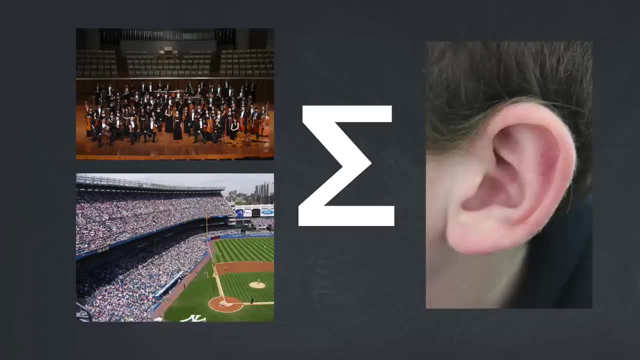 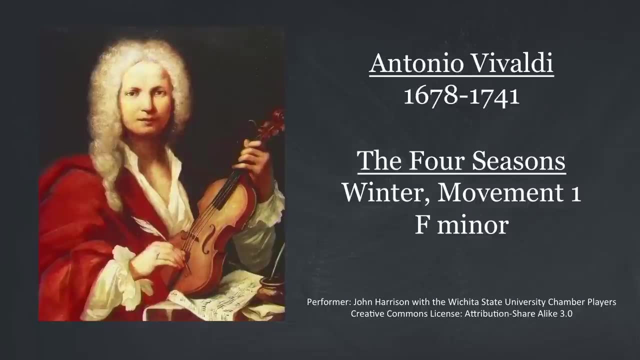 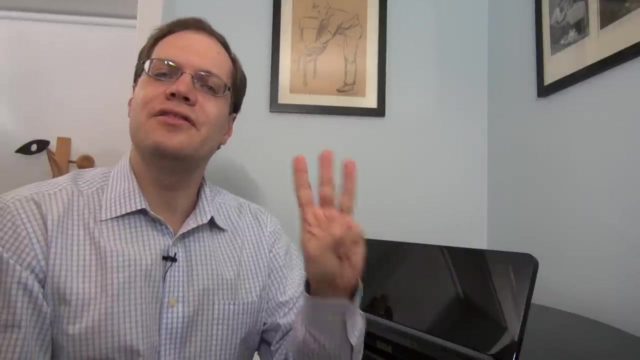 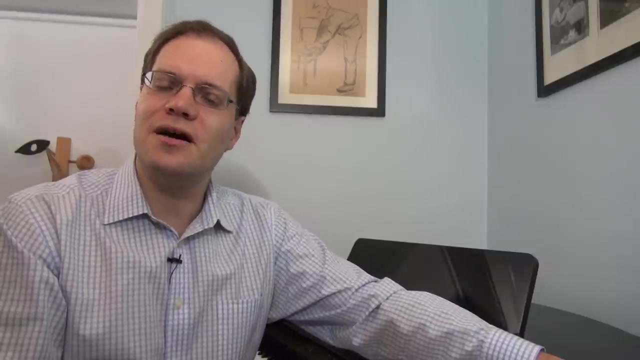 to extract those individual pieces. All right, so here is what we're going to do now. I will play three notes simultaneously on this piano, and I won't tell you what those notes are, but then we'll look at the resulting audio signal on the computer and by analyzing 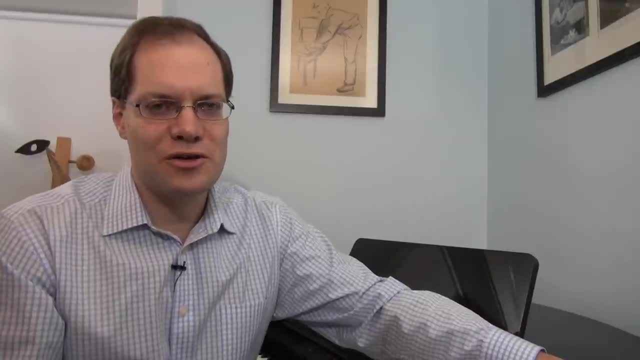 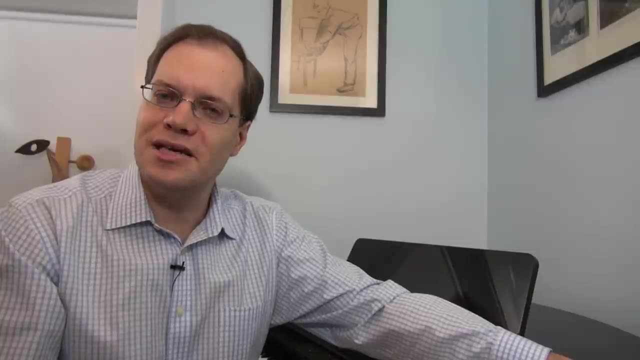 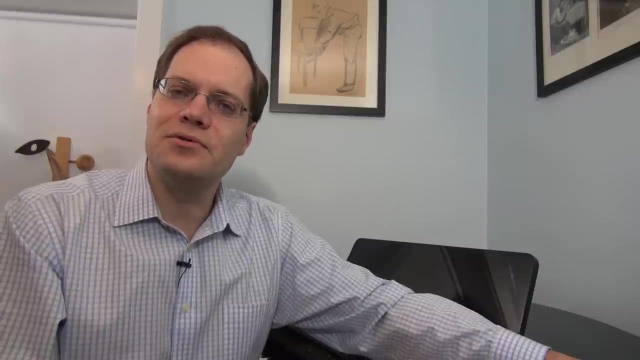 that signal, we'll try to determine what those notes were. So that's the task Now. because this is a digital piano, when I play those three notes at the same time, its internal logic will add the three signals together And then its speakers will play the resulting sum. 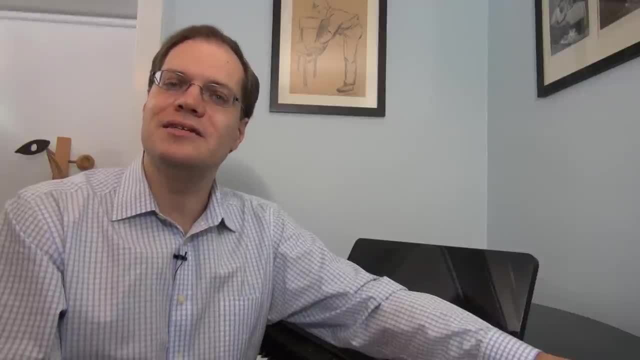 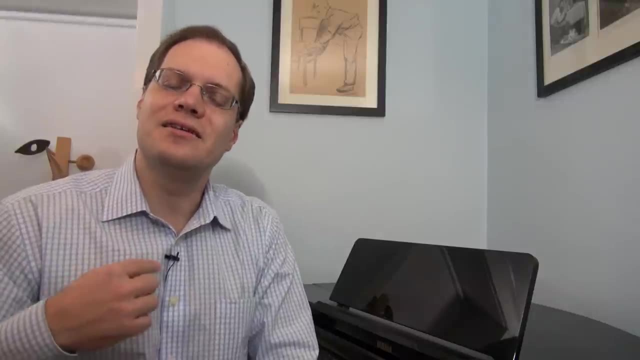 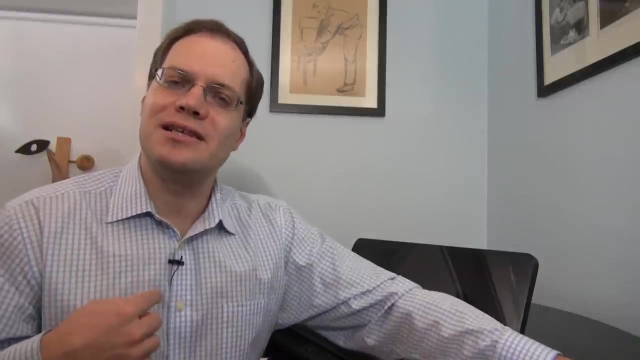 Had it been a real piano, then the three notes would sound individually, But then the laws of physics would add up the three signals together And in either case this microphone receives the resulting sum, And the task we're faced with is decomposing that one signal into the individual notes. 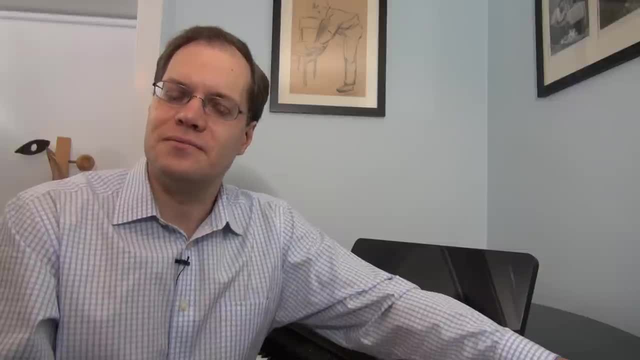 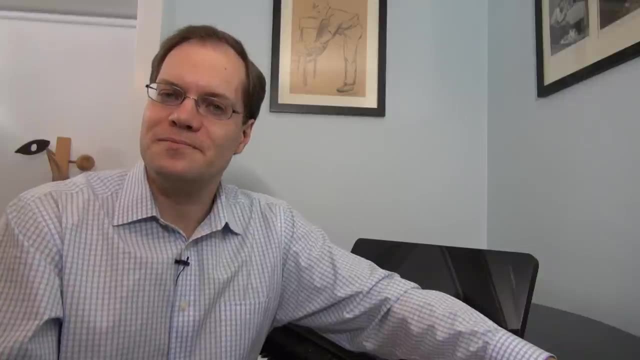 So the task that we're faced with is that of decomposition, Which is taking the resulting sum and determining what elements went into that sum and in what proportion. The problem of decomposition is the first and perhaps the biggest topic in linear algebra. 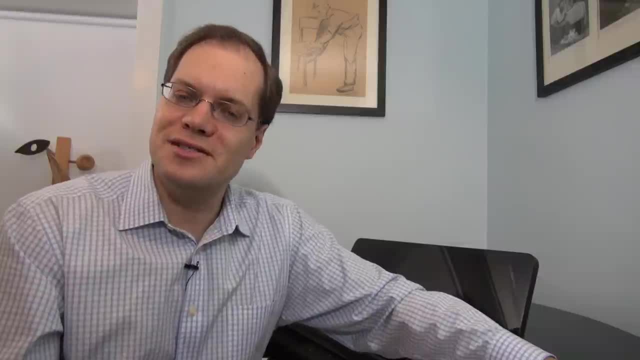 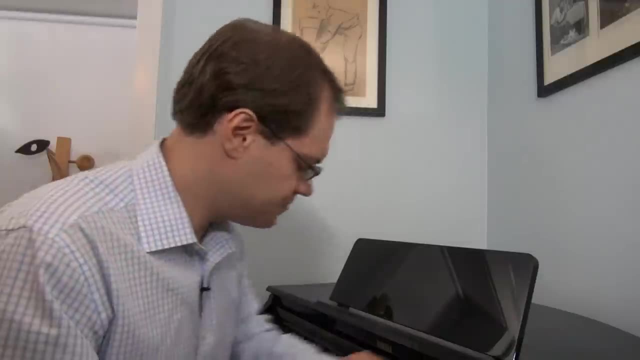 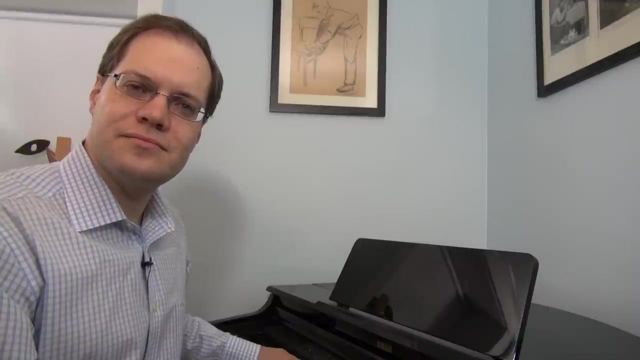 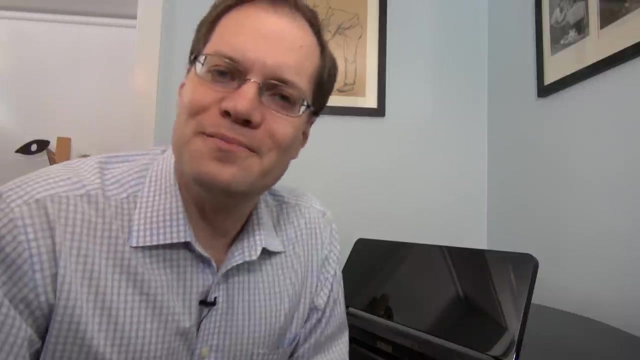 So it's a great place to start. So let me play those three notes at the same time, record the audio, and then we'll look at that signal on the computer. So here they are, Alright. so now let's walk over to the computer and look at the result. 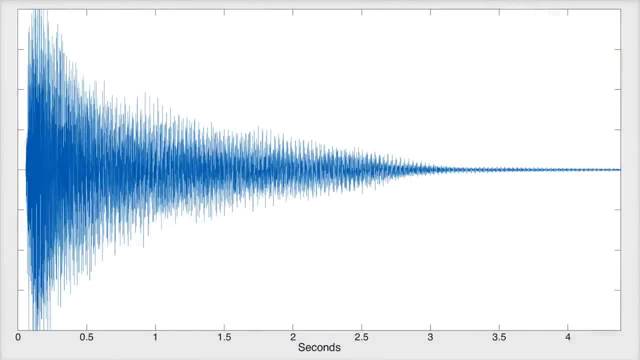 So we're now looking at the signal that we just recorded, And please notice that it's not three different signals representing three different notes. It is a single signal representing all the notes at once, And it's our task to somehow see the individual notes in this one signal. 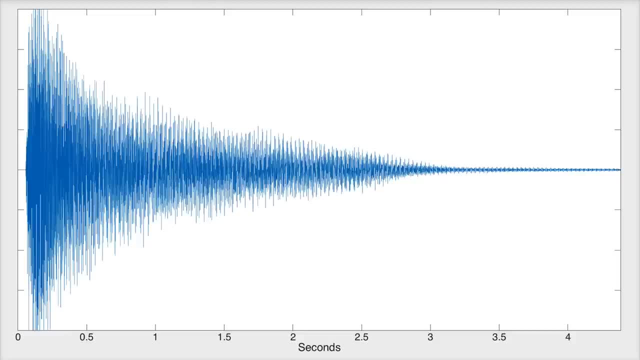 Each signal will act on a symbol that is completely different from each other. All of these signals have to be included, So how can I define a signal now? we're currently fully zoomed out and at this level of detail we can't say much, except perhaps that the sound starts out loud and then gradually dies. 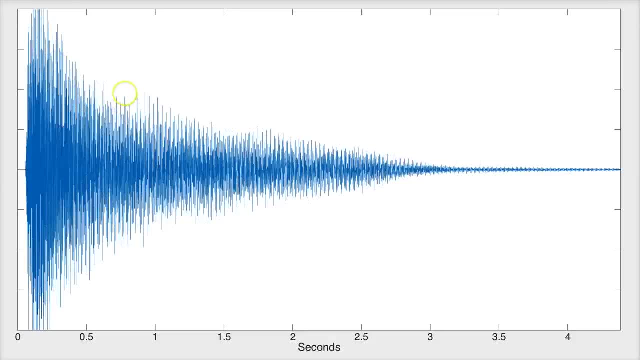 out and we're also seeing very subtle oscillations in volume, known as beats, and if you listen to the sound very carefully you will be able to hear those beats. but at this zoom level we don't have nearly enough detail to even begin determining the notes that were played. so let's zoom in on a very small part of 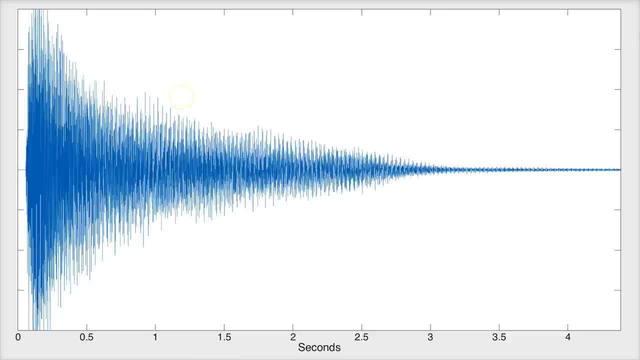 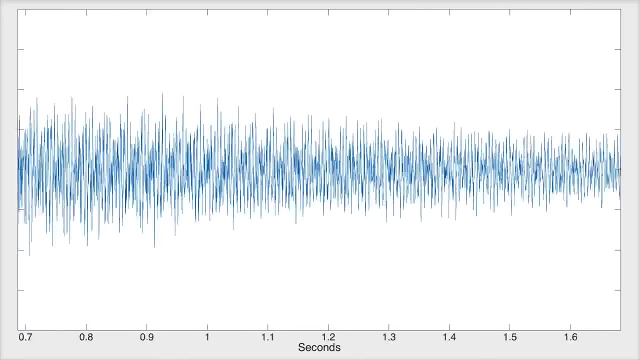 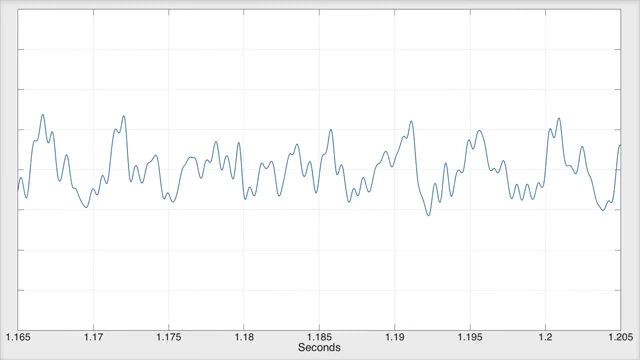 our signal right around here. that will give us sufficient detail to try and solve the problem we're facing. having zoomed in on four one hundredth of a second, we're finally seeing the complexity involved, and of course, it's this complexity that is responsible for storing such rich information in a single signal. so let's 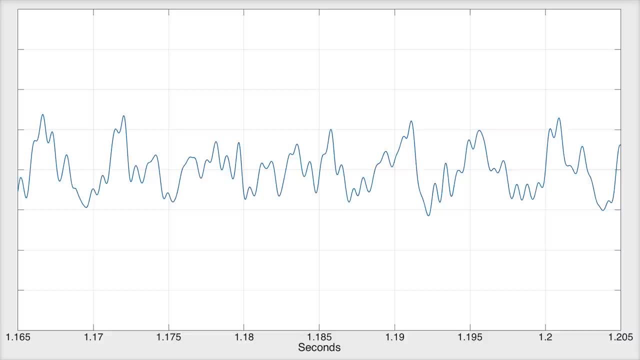 begin to analyze what we're seeing. what we're seeing is a signal that's somewhat periodic and that's characteristic of musical tones, and they're really two major features that our eye easily picks out. first of all, we're seeing these larger oscillations, of which there are one, two, three, four, five, six, seven. 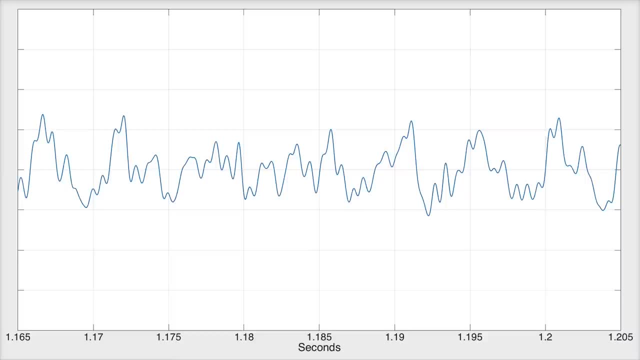 and on top of these larger oscillations we're seeing smaller, more frequent oscillations. that will count in a moment. but right there we just did our first bit of decomposition. we have looked at one thing and within that one thing we saw a sum of two different things, and those two things were the larger, less frequent. 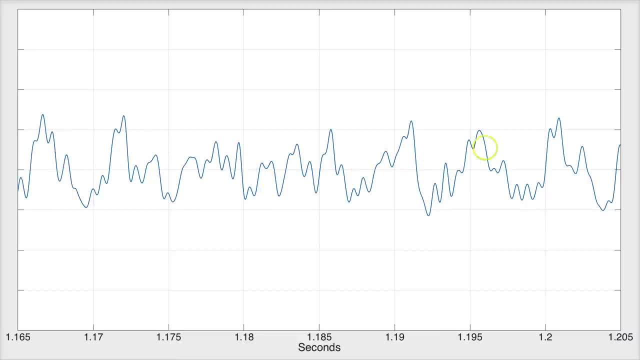 oscillations and the somewhat smaller, more frequent oscillations. so that, in a nutshell, is what we're seeing here: decomposition, seeing a single thing as a sum of two different things. let us now try to figure out what notes we're looking at, and that, of course, is. 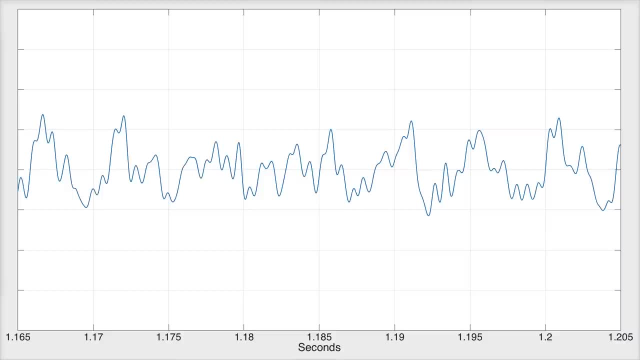 determined by the frequencies of these oscillations. now, there are seven of the larger oscillations in the four one hundredth of a second, which corresponds to 175 oscillations a second. in order to figure out what note this frequency corresponds to, let's refer to the 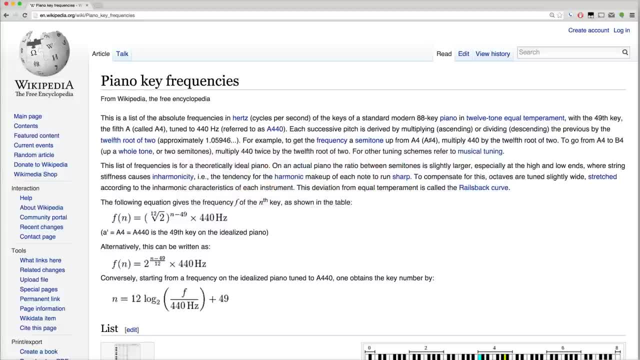 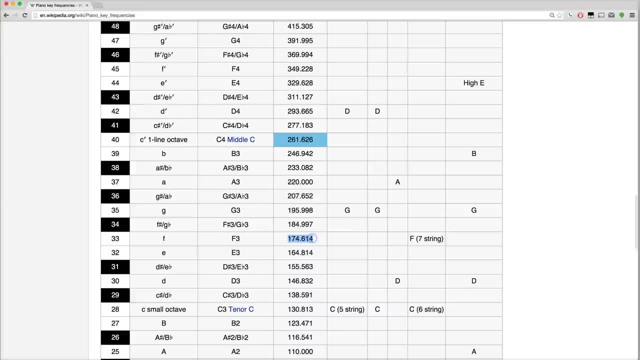 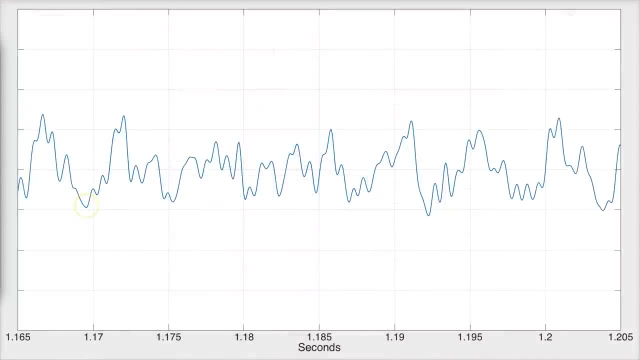 this Wikipedia article on the frequencies of musical tones and we find out that 175 corresponds to the F in the third octave Great. We have just determined one of the three notes. In order to identify another note, we have to determine the frequency of. 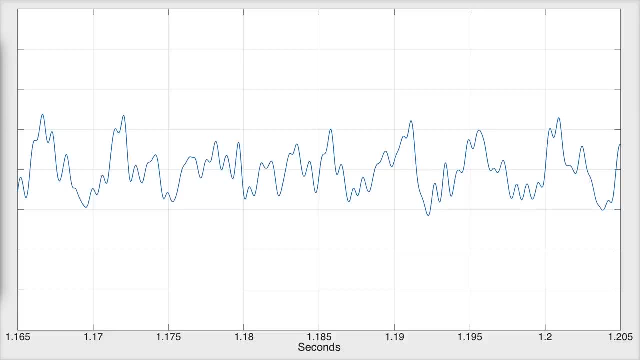 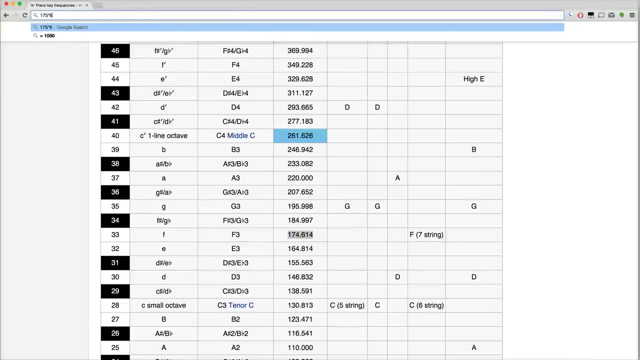 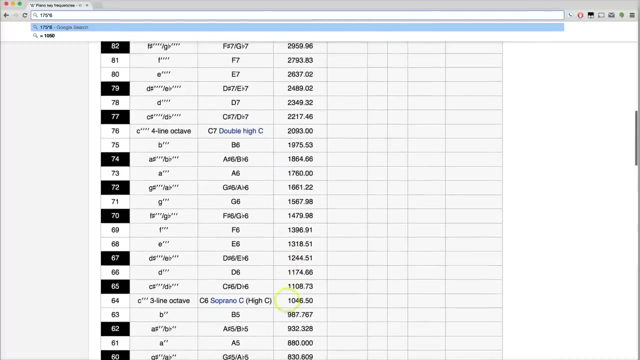 the smaller oscillations. Would you agree with me that there are roughly six of the smaller oscillations for each of the larger ones? That means that the frequency of the smaller oscillations is 175 times 6, or approximately 1050, which corresponds. 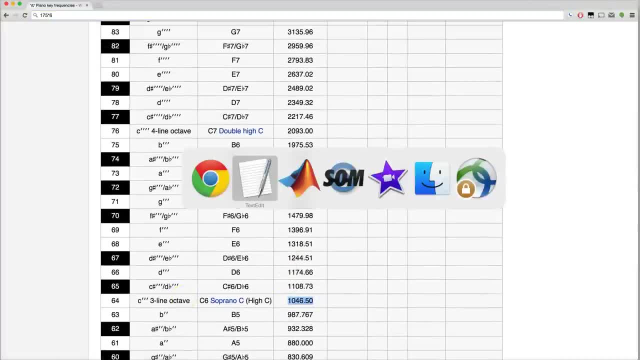 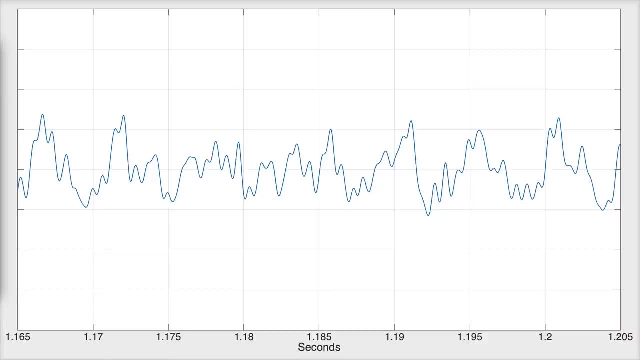 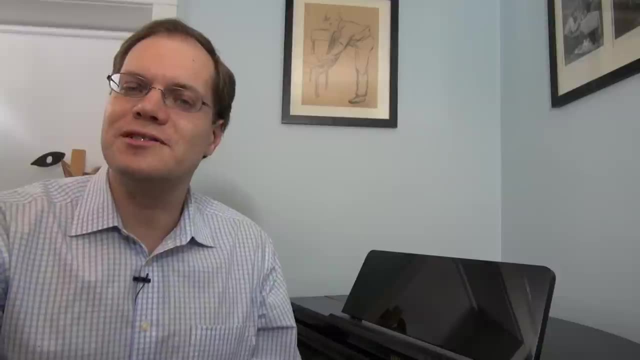 to the C in the sixth octave. We have therefore been able to determine two of the three notes, and I think that we are ready to go. I think that's about all we can do with the naked eye. So how well did we do? The answer is not bad at all. Let me reveal the notes that I had. 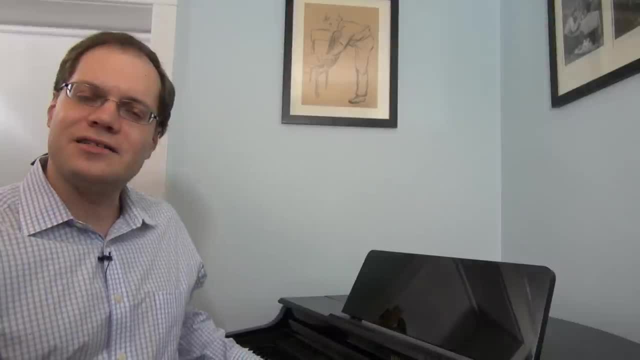 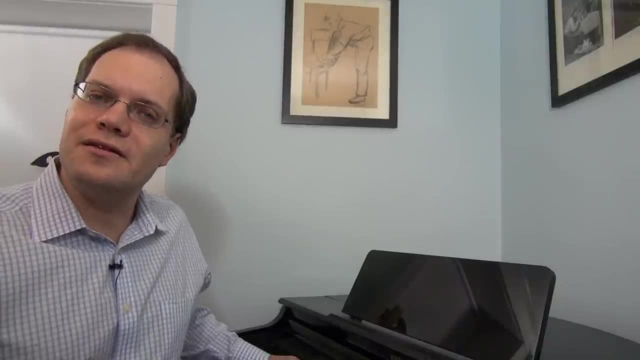 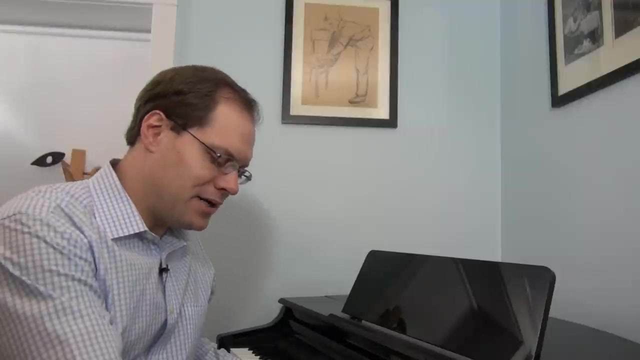 originally played. They were indeed the F in the third octave, followed by an A-flat and a C. Here they are all together, So we nailed this F Instead of this C. our eye picked out this C, which is a small mistake.